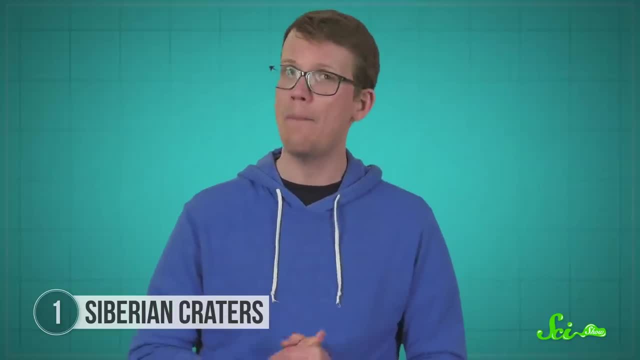 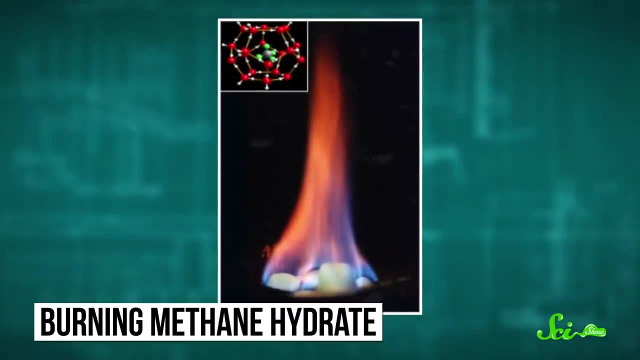 But no one's exactly sure where that gas is coming from, how pockets of it are forming or where the next one will be. One explanation is: this is all the result of melting methane hydrates, which form when methane gas is incorporated into the crystal structure of ice. 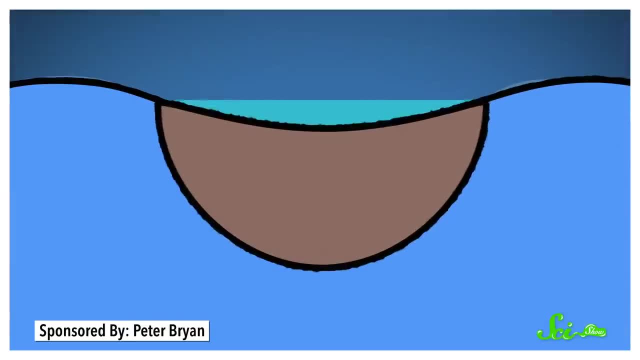 The methane itself is thought to come from deeper within the Earth. You see, when organic material buried long ago is subjected to extreme heat and pressure underground, it can produce methane, which rises up to the frozen permafrost, where it can get trapped in ice. 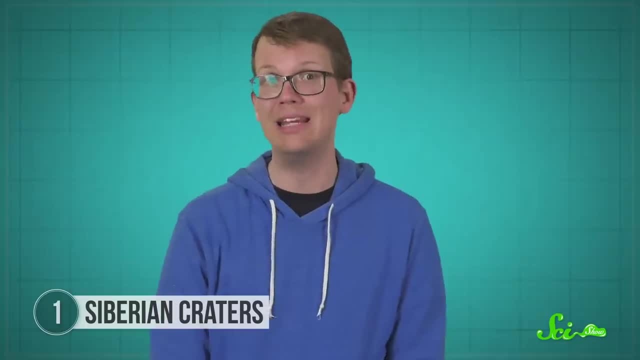 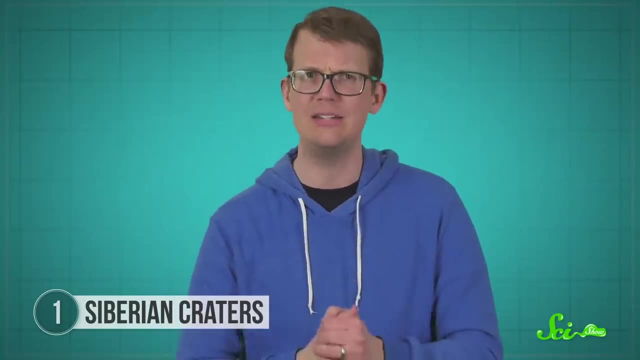 And if this is what's happening, then more explosions are probably on the way. With climate change warming the Arctic, methane hydrates are melting faster, But researchers are still debating the details here. Other studies blame microbes for the methane, And some don't think it's really about methane at all. 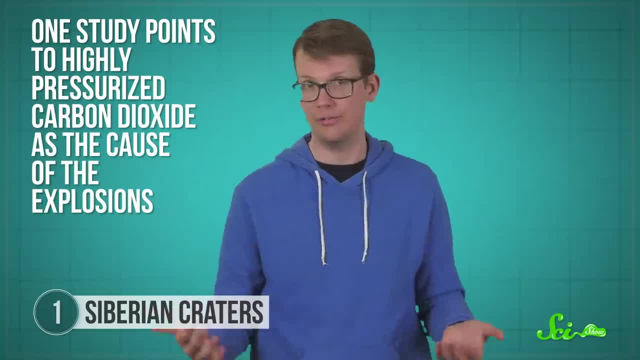 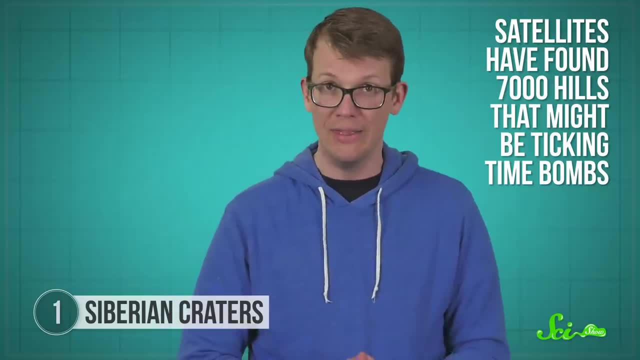 One study points to highly pressurized carbon dioxide as the cause of the explosions. And this is all critical to figure out, and you know fairly soon, because satellites have found 7,000 hills that might be ticking time bombs. Until we know what's actually happening, we will not know how many of these are dangerous. 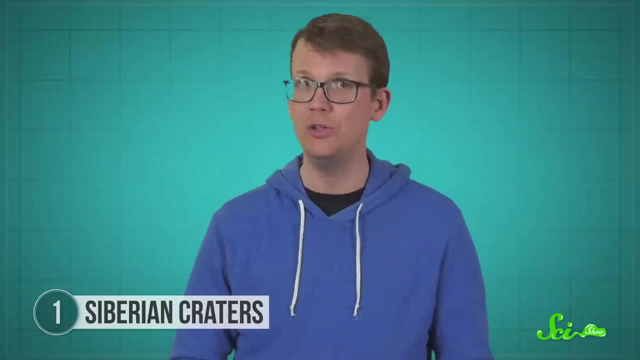 What we do know is that these hills form quickly over a few years, And studying them directly would probably shed some light on things. but they can be under very high pressure, so that's kind of tough. It's like when something is maybe about to explode. a researcher doesn't want to go out there and poke it to take a sample, Because what if you are the next crater? Explosions and impacts are two of the very few things that create near-perfect circles in the Earth, So circular features tend to be worth investigating. 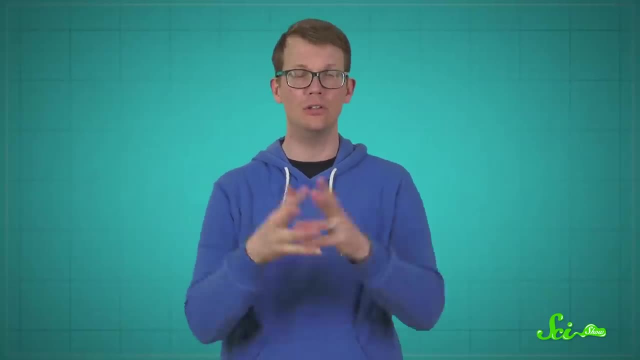 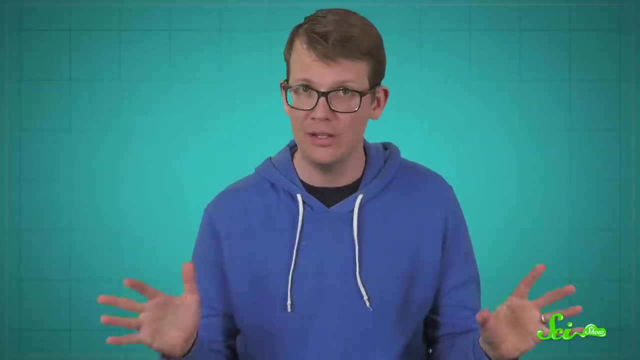 Well, it turns out, you've been looking at part of a near-perfect circle, at least by Earth standards. every time you look at a map of the world, And once you see this, you will not be able to unsee it. 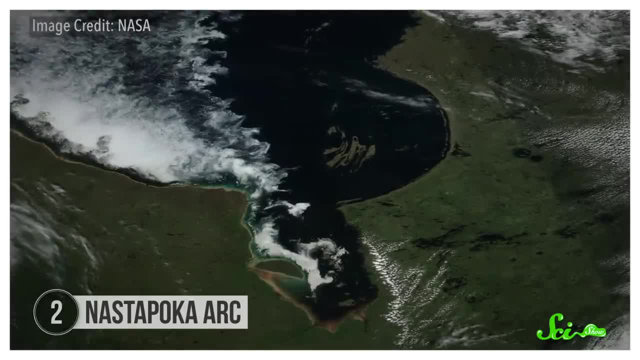 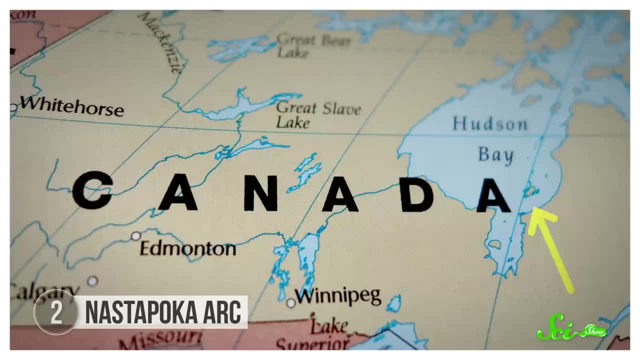 It's called the Nastapoka Arc. It's 650 kilometers long and makes up a big section of the Hudson Bay in Canada. Clearly, something big happened here. The first idea was that this is an impact crater, the site of a massive thing from space hitting the Earth. 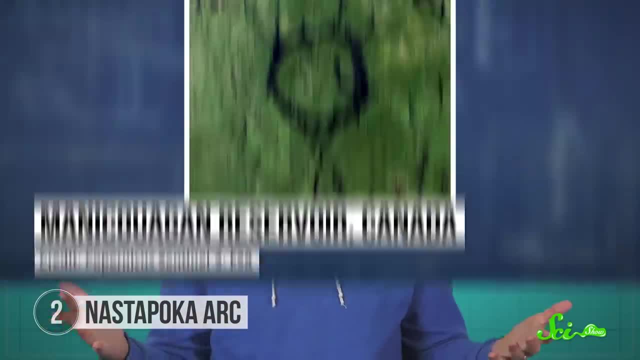 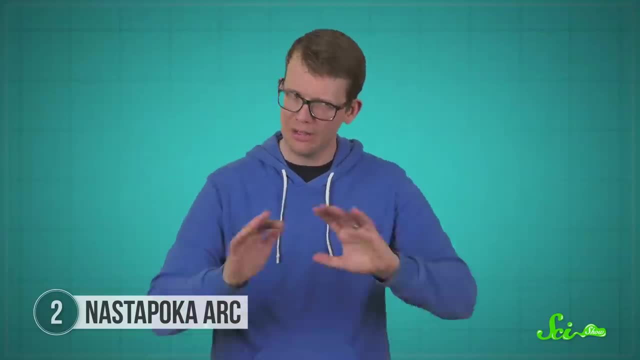 There are plenty of other circles that we know formed this way, like nearby Lake Manicougan, another circle on maps that you just won't be able to unsee. But when something slams into the Earth, it leaves behind a number of pretty telltale clues. 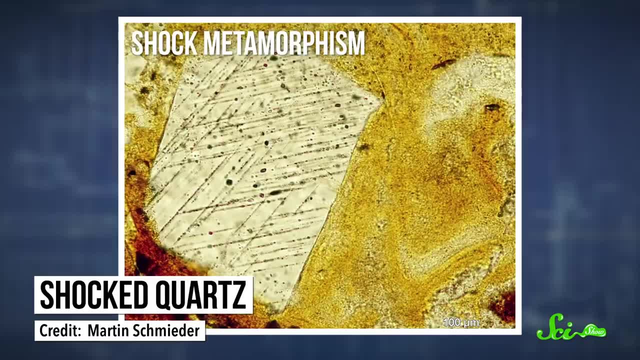 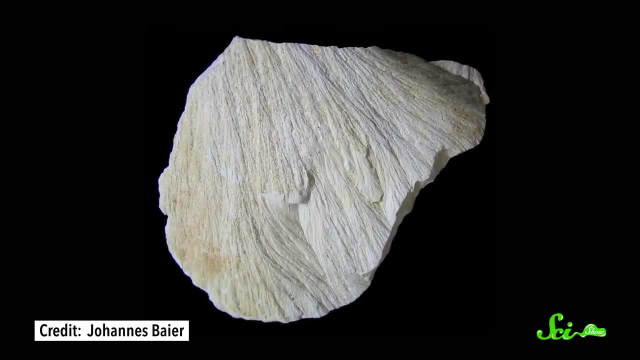 Things like weird rocks thanks to shock metamorphism, where heated pressure from a sudden impact deforms and even alters the minerals in rocks Or shatter cones, unique patterns of striations on rocks that only form beneath impacts, And the Nastapoka Arc doesn't have that. 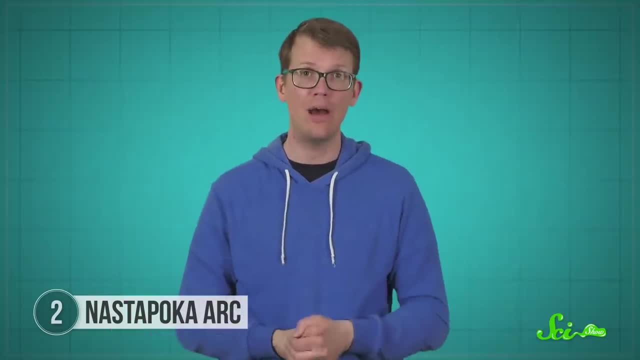 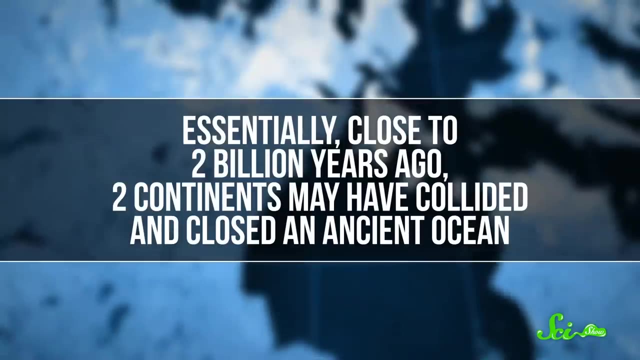 It doesn't have either of those. That's left scientists with one other hypothesis: that the curve was once the boundary between two tectonic plates, Essentially close to two billion years ago. two continents may have collided and closed an ancient ocean. 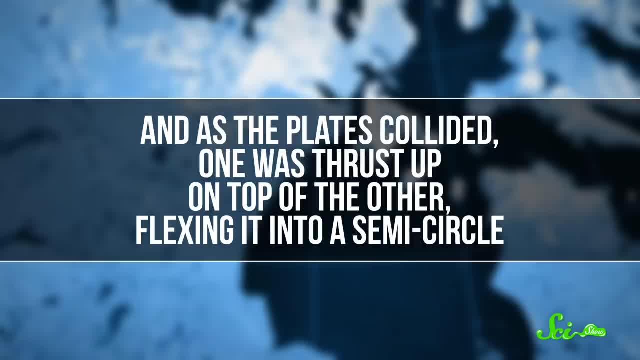 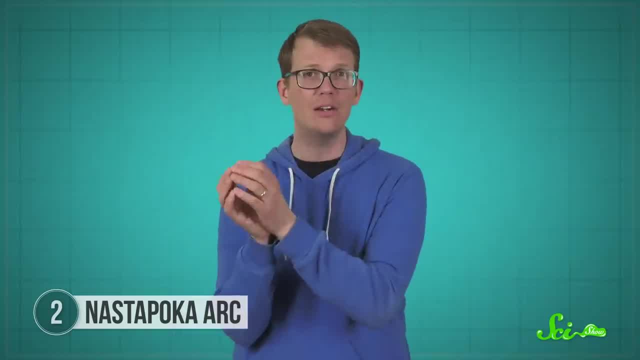 And as the plates collided, one was thrust up on top of the other, flexing it into a semicircle. But circular boundaries between plates aren't common. The idea is that here, as material from one piled up on the other, an unusually massive 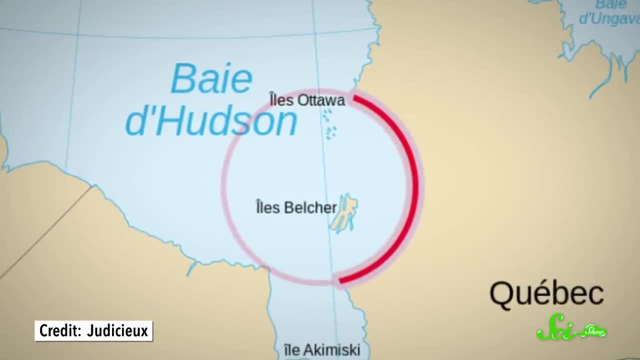 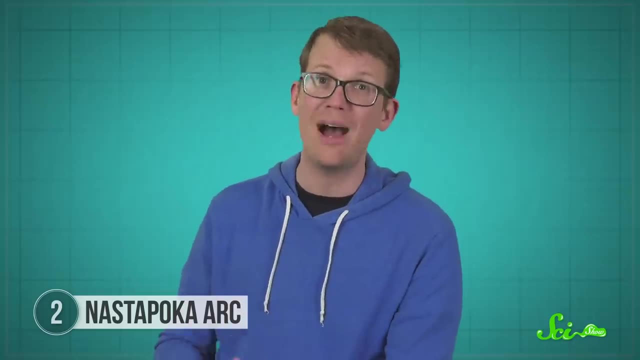 massive amount of rock built up in a relatively small area, the center of the circle we see today. The weight of all of that was so much that it pushed the lower plate down in a single spot, creating a semicircular bend in the crust. 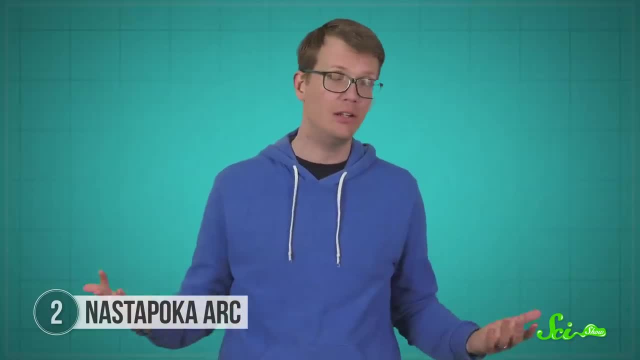 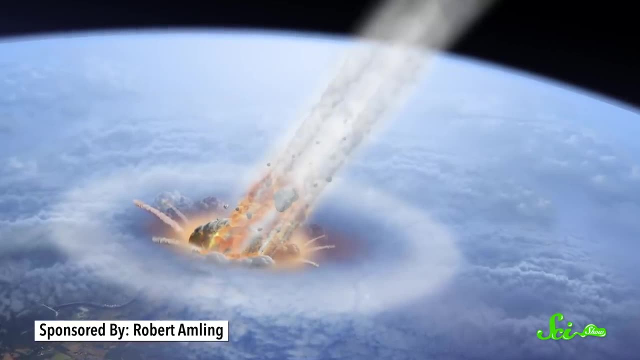 Now, while that could make sense, other areas where there have been similar plate collisions are not perfect circles, So some geologists still think that this was an impact, perhaps a really ancient one. so the usual evidence has been lost to time, And so we are left waiting for some adventurous geologist. 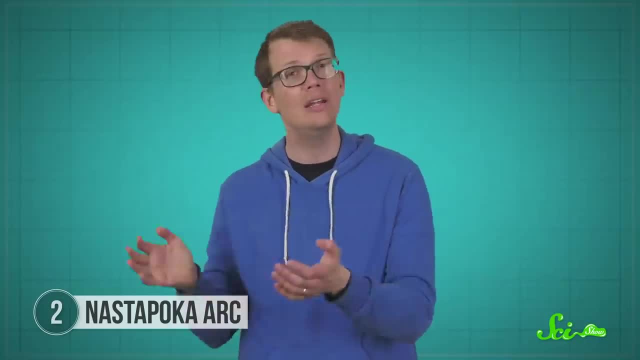 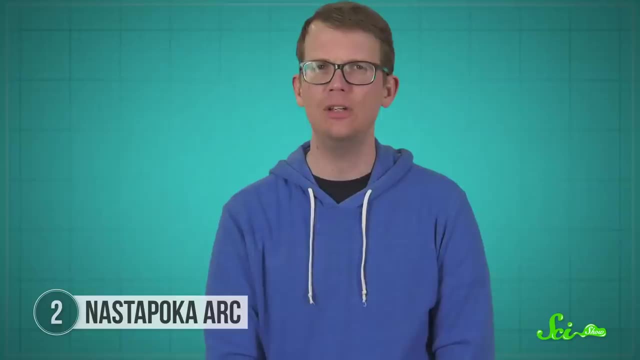 to find either clear evidence of an impact or a unique plate collision to close the loop on this very large, very mysterious circle. Now, not every mystery can be seen with the naked eye. A patch of the Indian Ocean is missing gravity, and no one's entirely sure why. 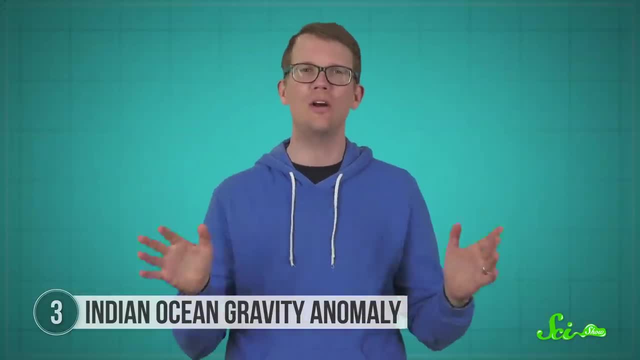 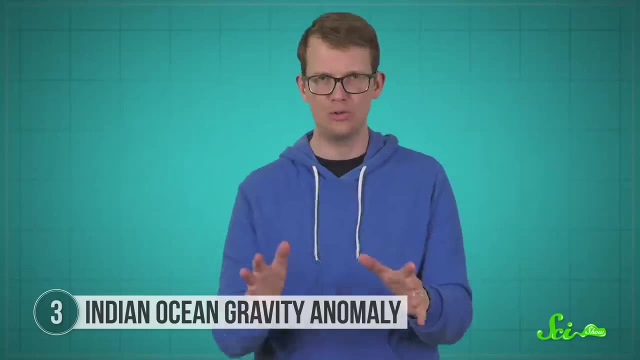 Now it's not that you can like go here and float. You couldn't even jump any higher if you were standing on a ship there. These are tiny differences that geophysicists detect with very precise instruments. Studying Earth's gravity at different places allows us. 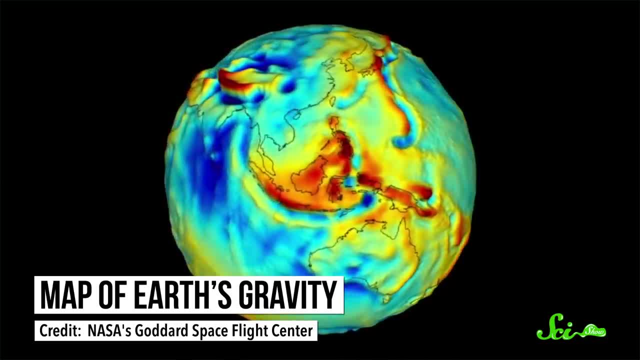 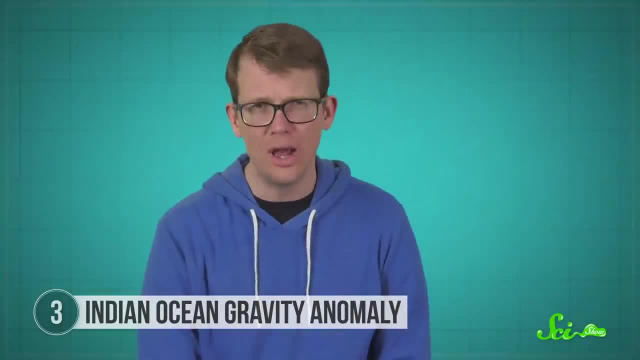 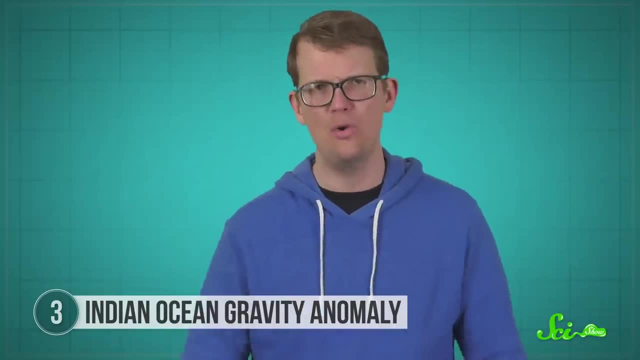 to see beneath the surface of our planet. See higher gravity means that something is more dense down there, and vice versa for lower gravity. Except that Earth scientists are totally stumped by the largest gravity anomaly of them all: a massive spot of low gravity in the middle of the Indian Ocean. 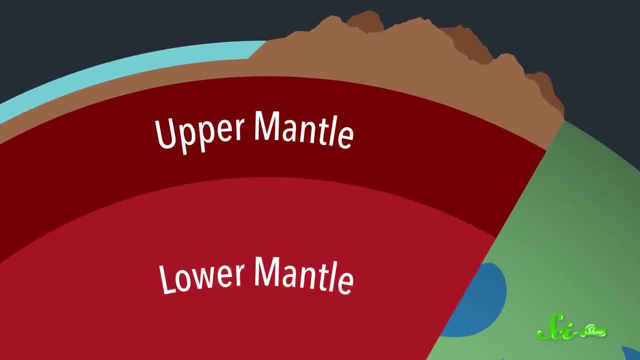 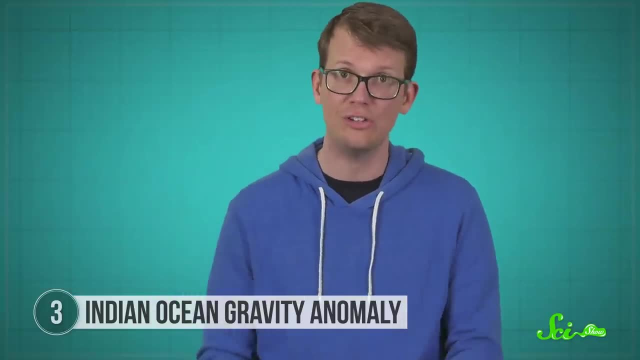 It could be that the mantle isn't the same in every spot and there's a plume of hotter, less dense material down there, But some think it goes all the way down through the planet's mantle, essentially suggesting there's a… a dent in the mantle. 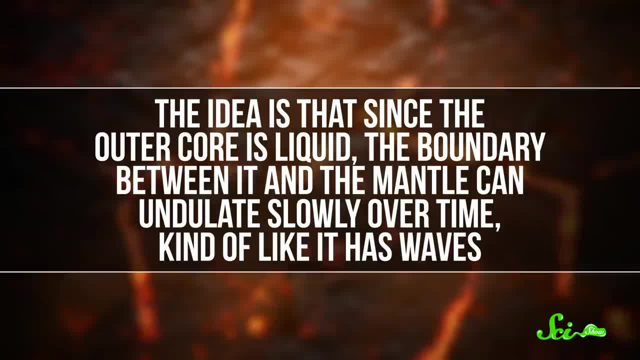 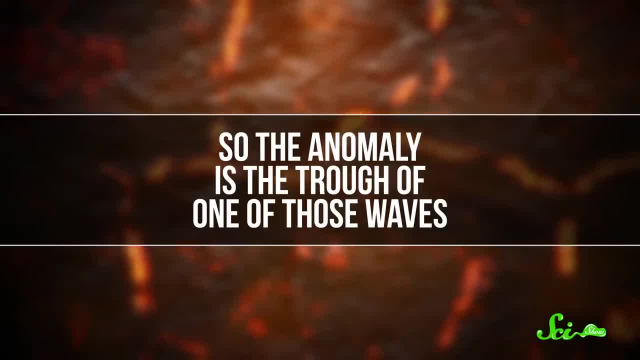 The idea is that since the outer core is liquid, the boundary between it and the mantle can undulate slowly over time, kind of like it has waves. So the anomaly is the trough of one of those waves. Others think there are slabs of old continents sitting down there. that 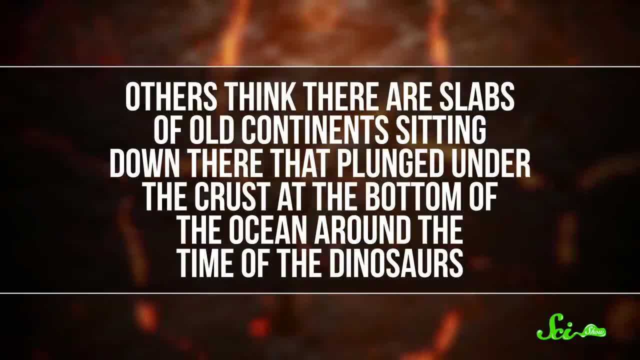 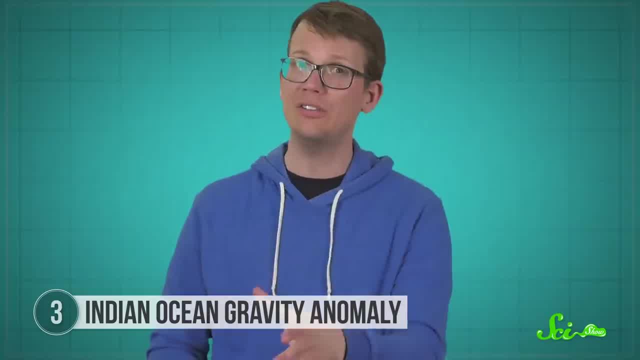 plunged under the crust at the bottom of the ocean around the time of the dinosaurs. Researchers are still learning about what happens to tectonic plates after they've sunk beneath the crust, But it turns out they can take hundreds of millions of years to mix back up. 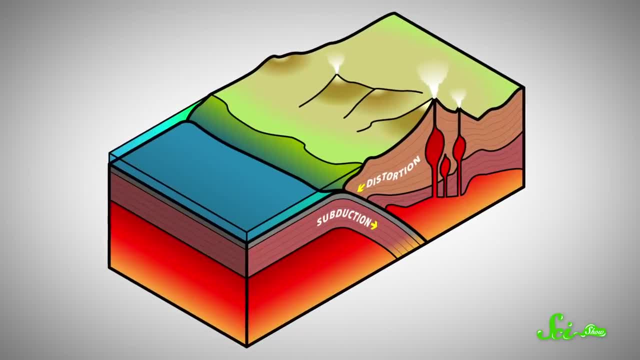 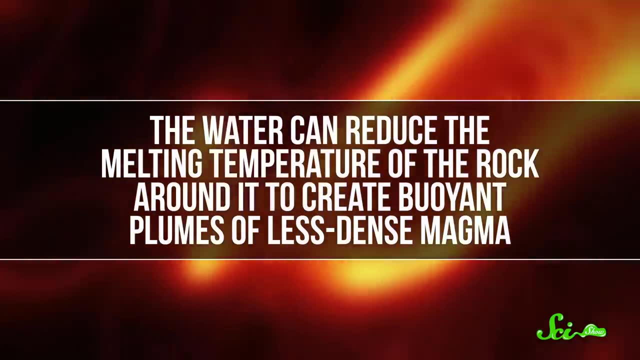 And the hypothesis here is that these subducting slabs bring water down with them. The water can reduce the melting temperature of the rock around it to create buoyant plumes of less dense magma, and those could be responsible for the low gravity at the surface. 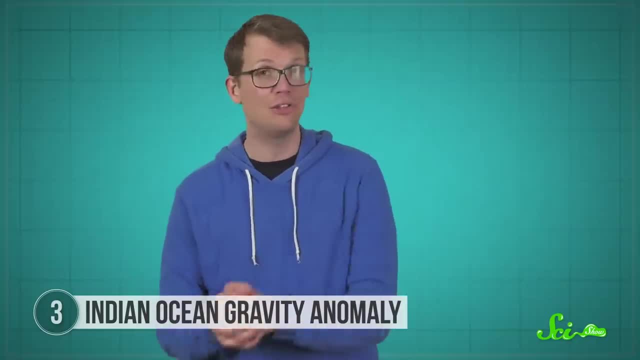 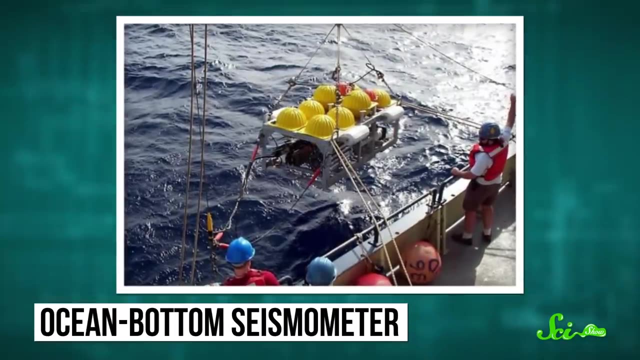 There's certainly no shortage of ideas, but determining which one is the right one will require some higher-quality images of what's going on beneath the seafloor, And that's why geophysicists have stuck a bunch of seismometers in the middle of the ocean. 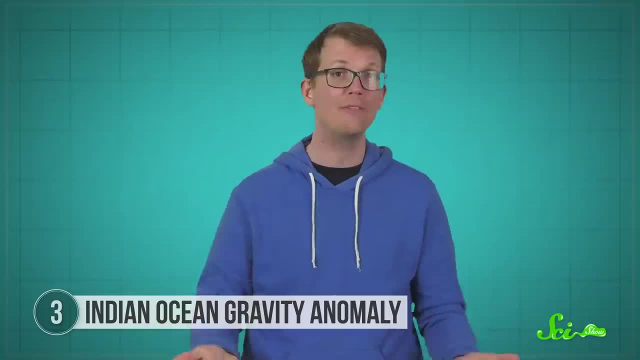 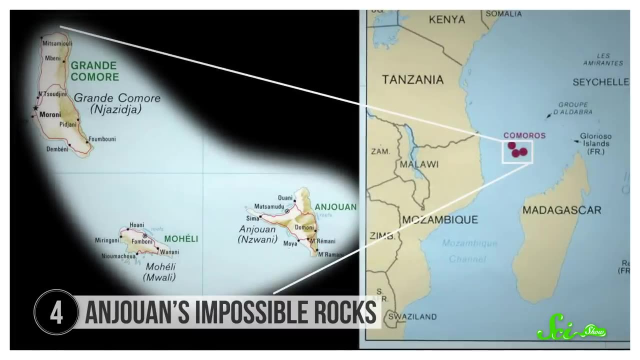 They're hoping the way seismic waves from earthquakes interact with whatever is down there will give them clues to what's really going on. Our next mystery takes us to the small island of Anzouan off the northern coast of Madagascar. See, this island has the wrong type of rock on it. 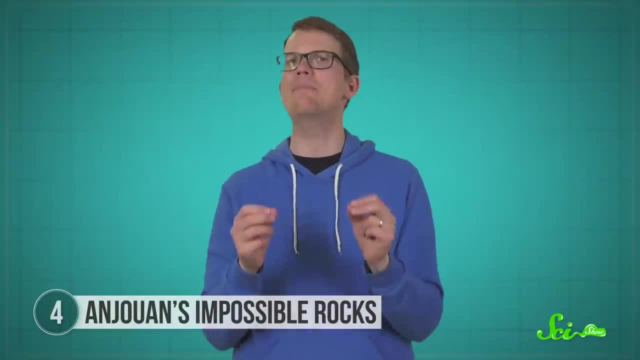 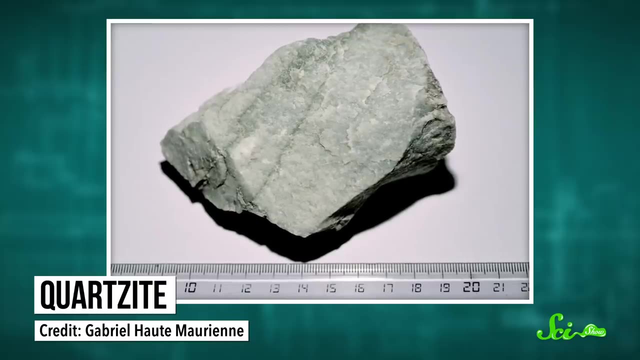 And by that I mean it is an unexpected type of rock. You see, Anzouan is a volcanic island, but on its surface you can find a rock called quartzite Which, frankly, it just should not be there. 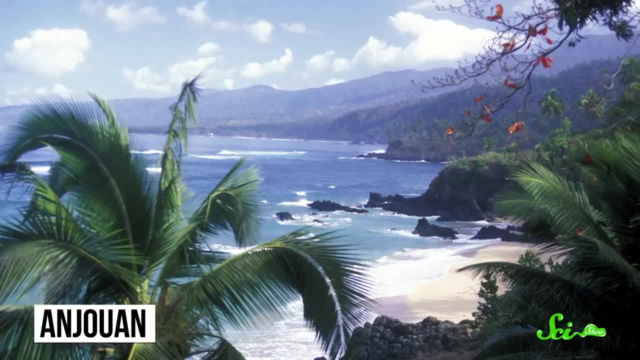 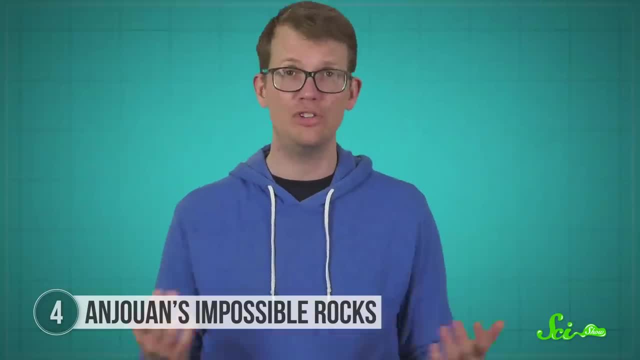 It's pretty clear how the island itself formed: An undersea hotspot. volcano slowly built up rock until it made an island similar to the islands of Hawaii. And this one is relatively young, by geologic standards, around 4 million years old. And all of this makes Anzouan the last place you would expect to find quartzite. 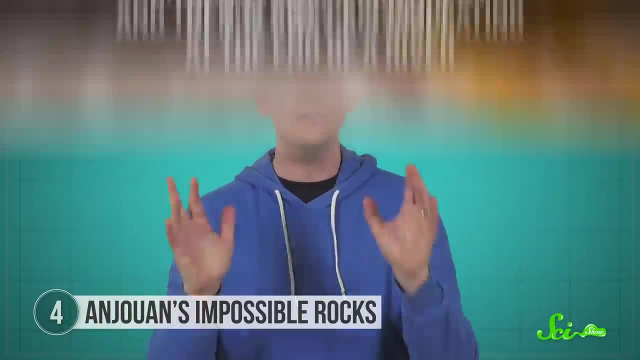 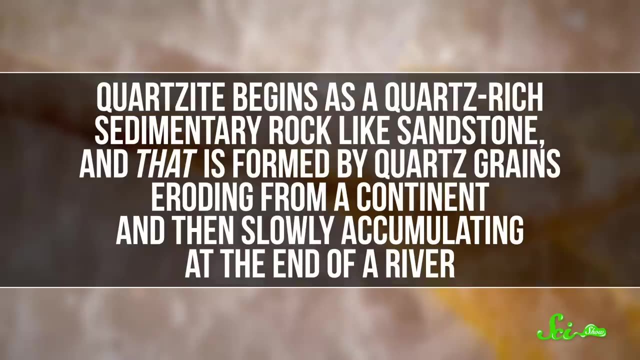 Now that requires some explanation, but not a lot of explanation, because quartzite begins as a quartz-rich sedimentary rock, like sandstone, And that is formed by quartz grains eroding from a continent and then slowly accumulating at the end of a river. 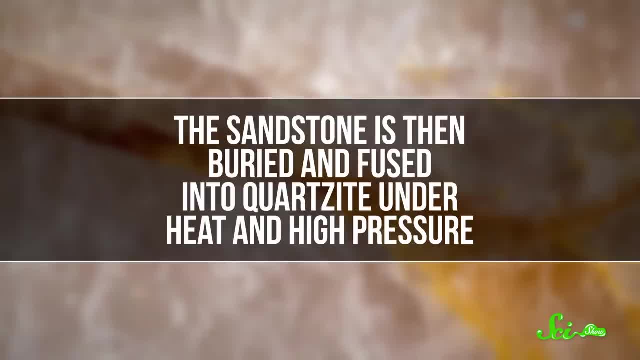 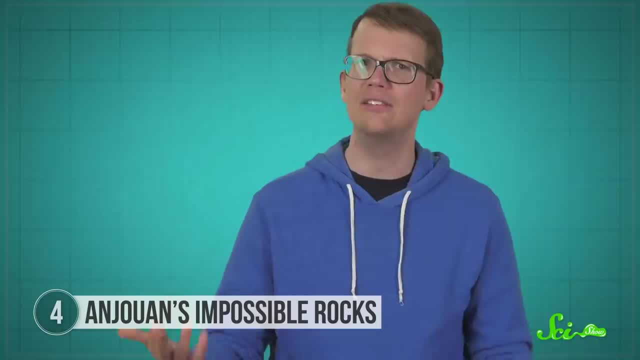 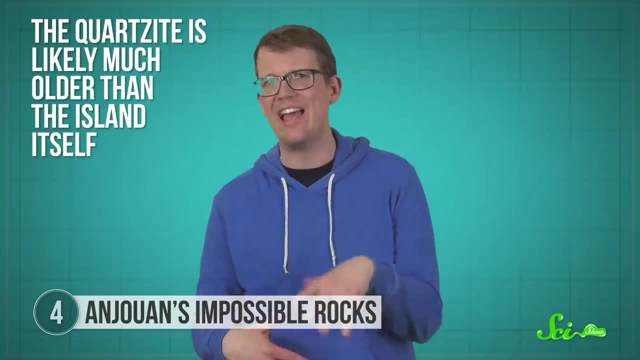 The sandstone is then buried and fused into quartzite under heat and high pressure. And that's the mystery here: The quartz shouldn't have eroded from the volcanic rock of the island itself. It must have come from some larger continent. And besides all of that, the quartzite is likely much older than the island itself. 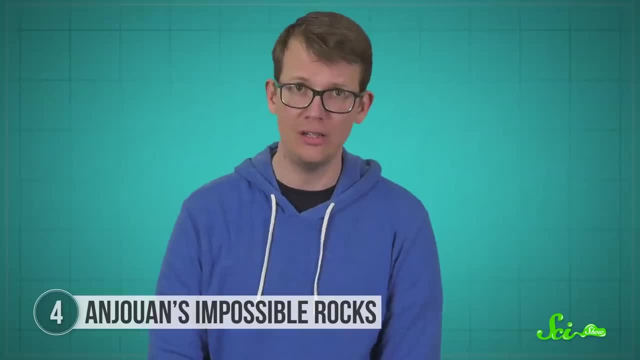 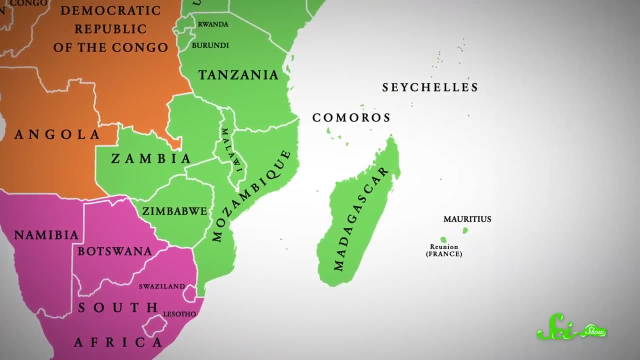 They've been dubbed the impossible rocks by the researchers studying them, and their history is still very much an unanswered question. The current hypothesis is that they came from the African continent, possibly when Madagascar broke away, but it's not clear how this would have happened. 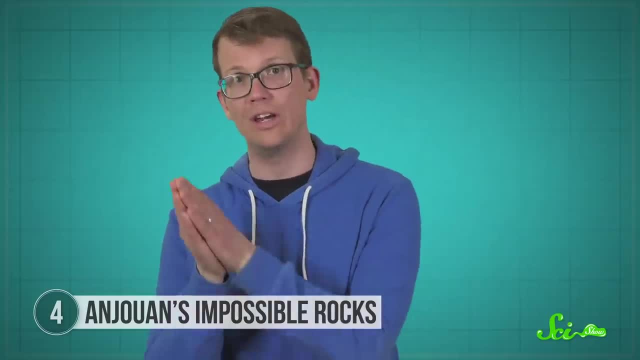 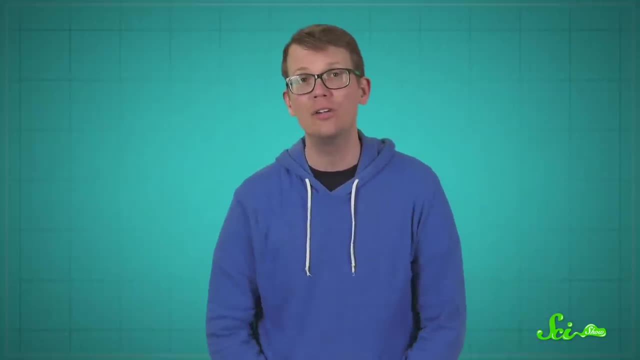 So the next step for the researchers is to figure out exactly how old the quartzite is and compare it to the age of rocks in East Africa and Madagascar to see if they find a match. One of the most long-standing geologic mysteries is also one of the most seemingly mundane. 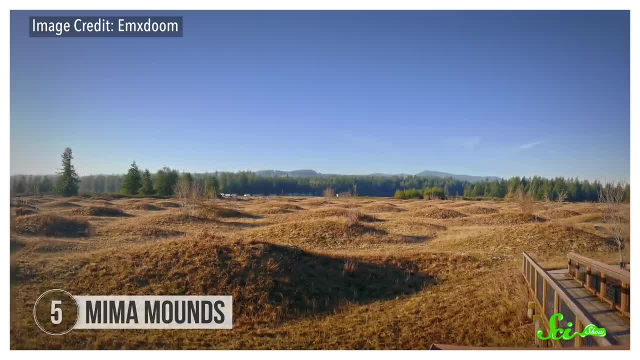 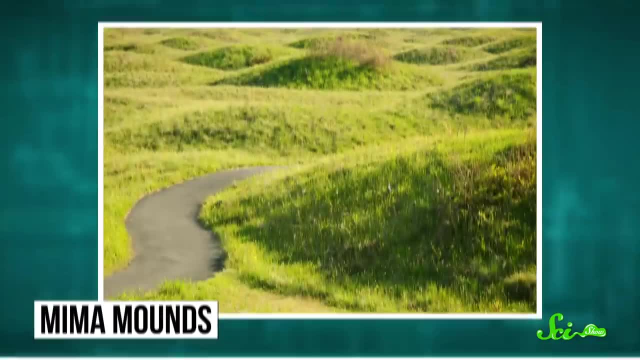 Mima mounds might not look like much at first. They're just mounds of sediment most famously found in Washington state. though similar formations exist. They exist on every continent except Antarctica. Each can be between 2.5 and 15 meters across and up to 3 meters high. 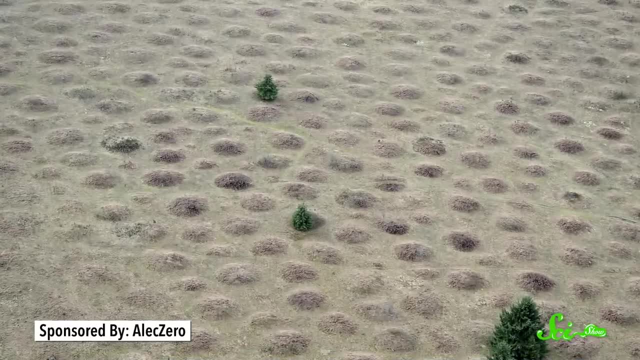 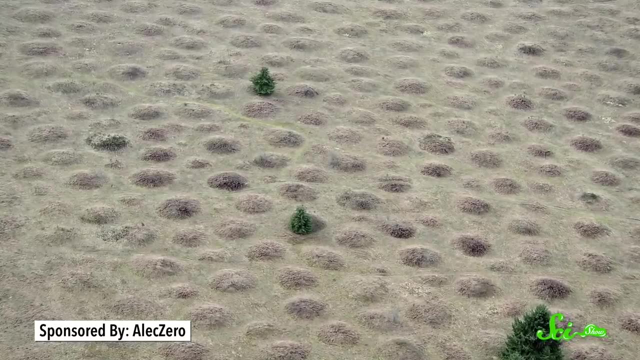 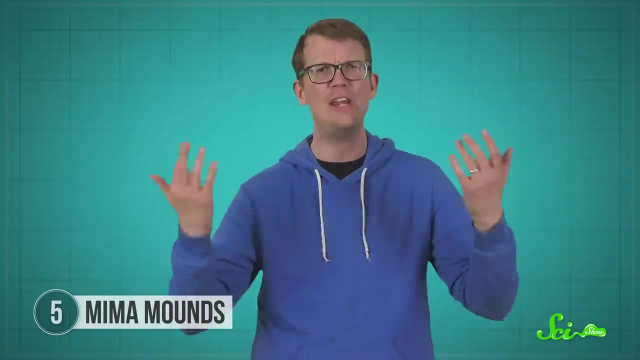 So like they're just not super impressive features. Still, these little bumps have been haunting the dreams of geologists for almost 200 years. We simply don't know how they form. There have been over 50 explanations proposed, everything from earthquakes shaking the sediment to winds building them during droughts to insects. 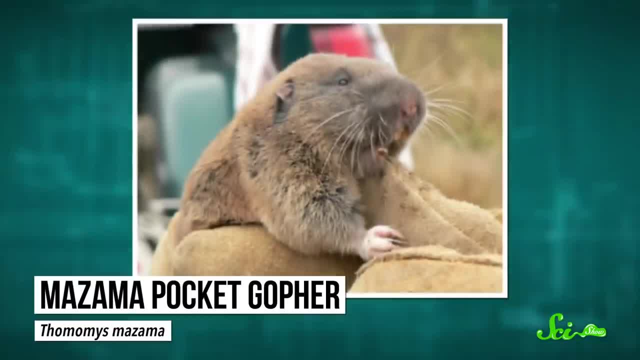 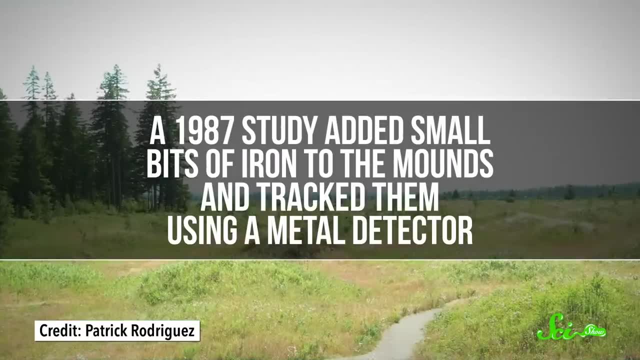 slowly constructing them, bit by bit. In 1942,, scientists proposed that pocket gophers were responsible And, believe it or not, that is still the leading theory to this day. A 1987 study added small bits of iron to the mounds and tracked them using a metal detector. 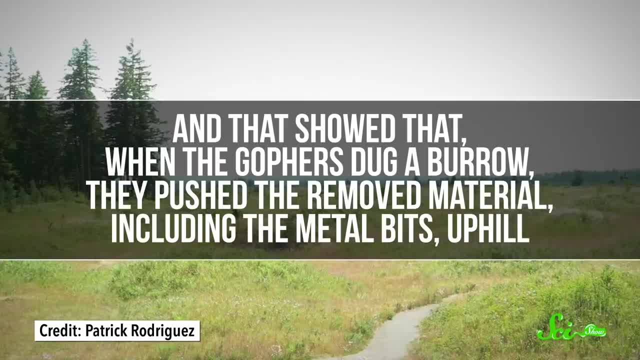 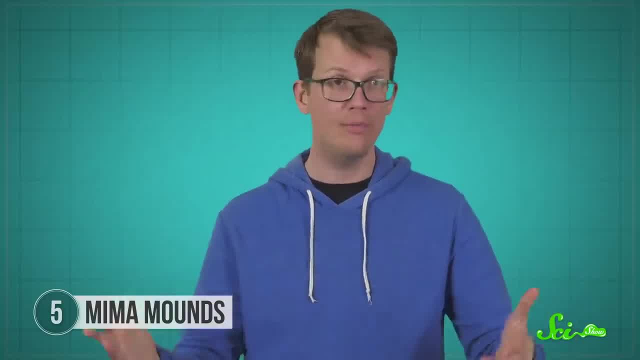 And that showed that when the gophers dug a burrow, they pushed the removed material, including the metal bits, uphill. Then, in 2013,, a computer model took those results and extrapolated them over hundreds of years And, at least according to the math, these wee gophers could build that kind of mound eventually. The process is predicted to take hundreds of years. an amazing multi-generational project for the little rodents. We still don't know why the gophers would do this, though. After all, it takes more energy to push sediment uphill when you're digging a burrow. Also, a model is far from conclusive proof, so other ideas could end up being right. So what we really need is for someone to take two flat areas of land. 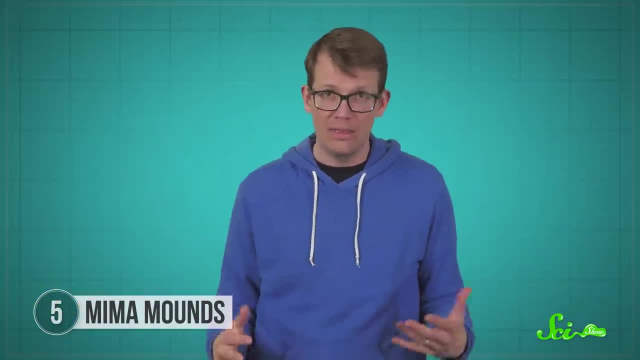 stick some gophers in one and keep gophers out of the other and then see what happens, And see what happens over about 500 years. You know, just some simple, straightforward science that we'd all be long dead before we got the results of. 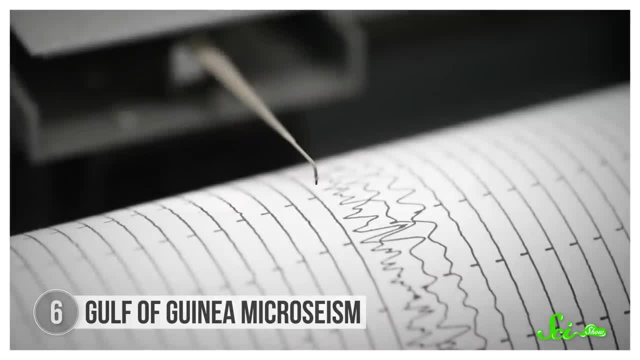 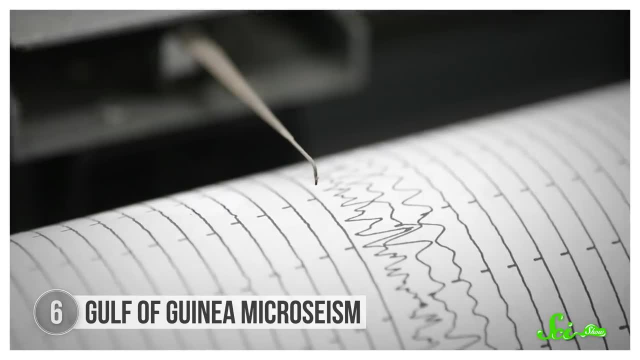 Our final mystery is that every 26 seconds, like clockwork, the Earth rumbles. Seismometers first heard this strange faint pulse called a microsism in 1961. Since then it has been detected all over the world except, strangely, not in South America. 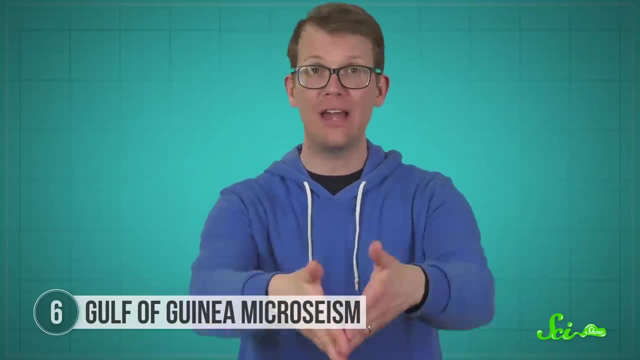 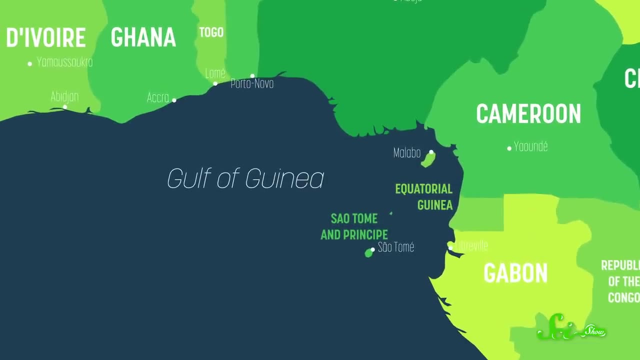 By comparing the signals at different seismic stations, scientists have triangulated the signal's origin. This leads to two spots. The strongest signal from the 1961 pulse was attributed to the Gulf of Guinea in the Atlantic Ocean, off the coast of Nigeria. 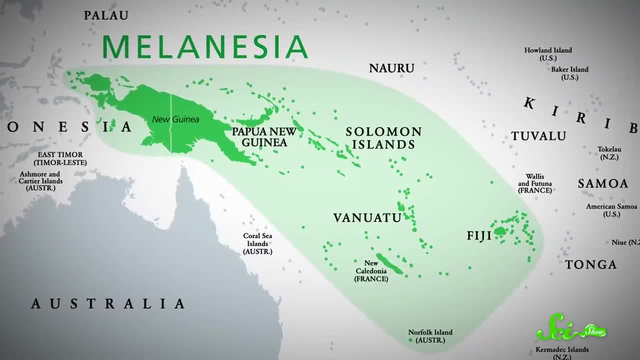 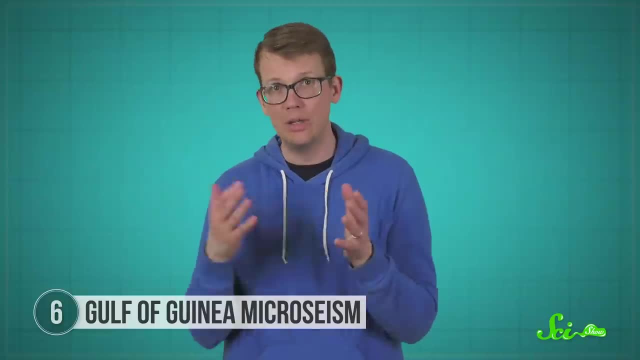 The second is in the Western Pacific Ocean near Fiji, But that is on the other side of the Earth. It's actually exactly on the opposite side of the world from that first spot. So scientists think that it could be originating in the Gulf of Guinea. 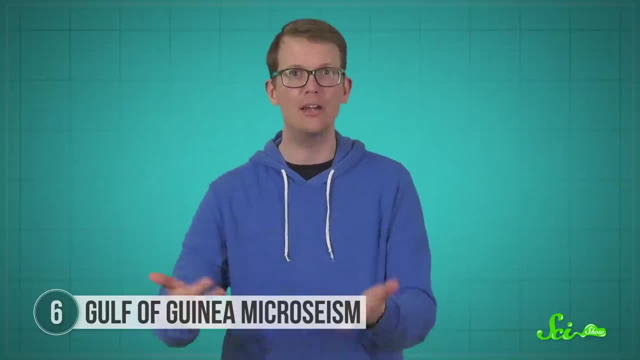 and then the seismic waves are traveling across the entire planet and concentrating on the other side. But no one is sure what the ultimate source is or why it occurs at such regular 20s. Some studies suggest it could be related to some part of the volcanic process. 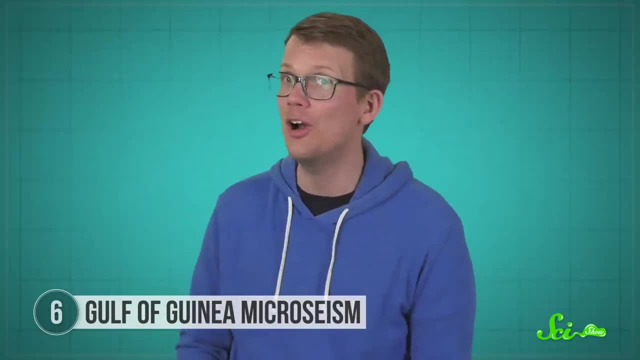 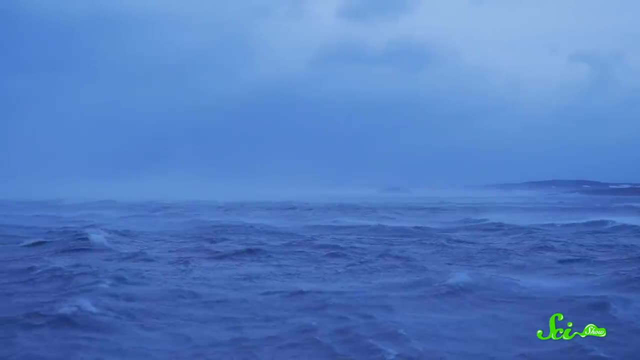 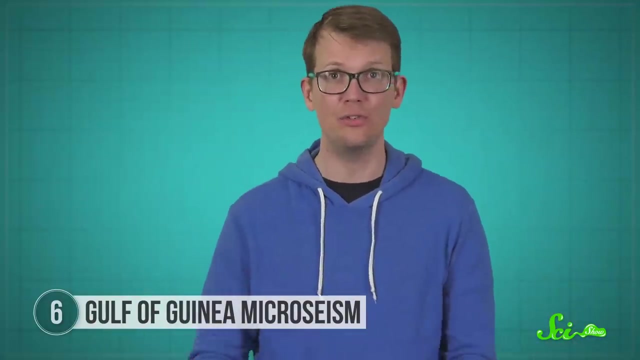 deep beneath the surface, But that wouldn't explain why it is stronger during storms and overall stronger when it's winter in the southern hemisphere. Instead, those both suggest it has something to do with waves in the ocean. Some experts hypothesize it's simply that the African continental shelf 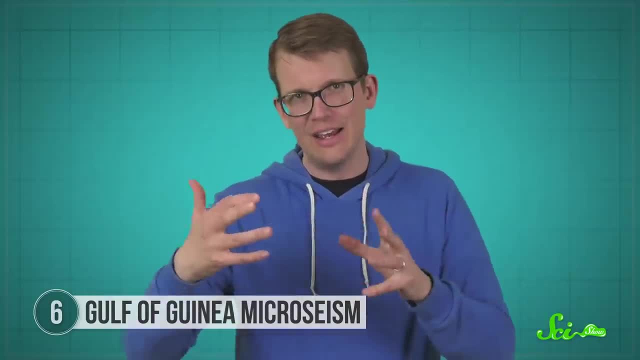 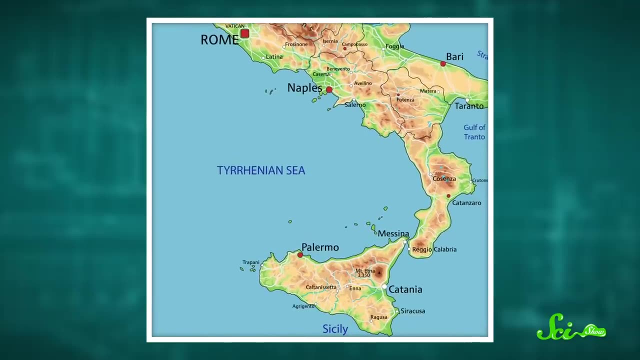 is shaped in such a way that, when waves hit it, they rumble through the Earth. A similar, though less impressive, rumble coming from the seas around Sicily was tracked down to ocean waves by comparing seismometers to wave data from buoys in the ocean. 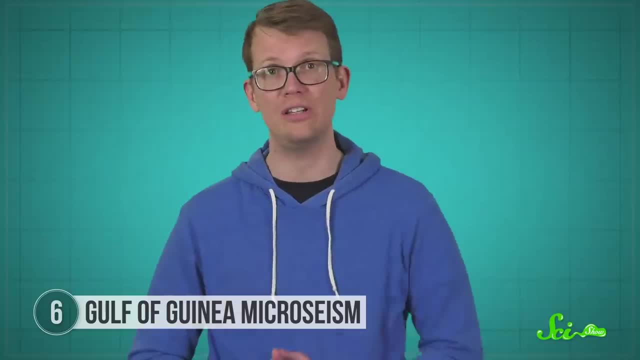 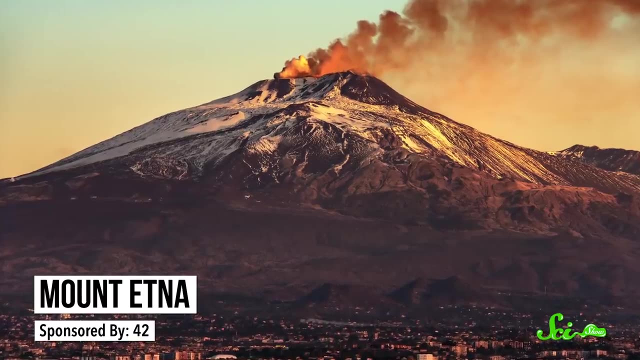 So that kind of setup could perhaps shed some light on this 26-second pulse. But the Italian rumble was conveniently close to Mount Etna. That meant researchers were able to repurpose an array of seismometers that was already there to monitor the volcano. 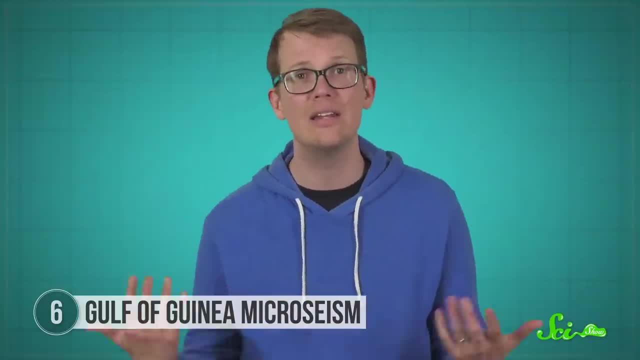 Nothing like that exists in the Gulf of Guinea area now, so getting the data needed to support the wave theory won't be so easy. Still, regardless of the data, it's still possible that the wave theory could be used to track down seismometers.